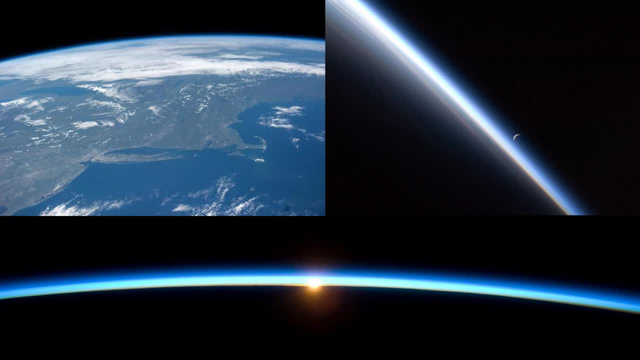 in this lecture and the next, we'll explore the answers and we'll learn why the other terrestrial worlds ended up so different, despite having formed under similar conditions. We'll also discuss why Earth's climate remains relatively stable and how human activity may be threatening such stability, with potential consequences that we are only now beginning. 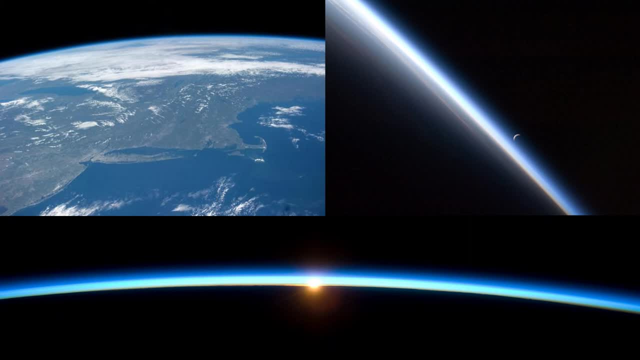 to understand, An average apple is about 225 millimeters around and its skin is about 3 millimeters thick. If we compare the Earth and its atmosphere to an apple and its skin, the skin of the apple is about 20 times thicker relative to. 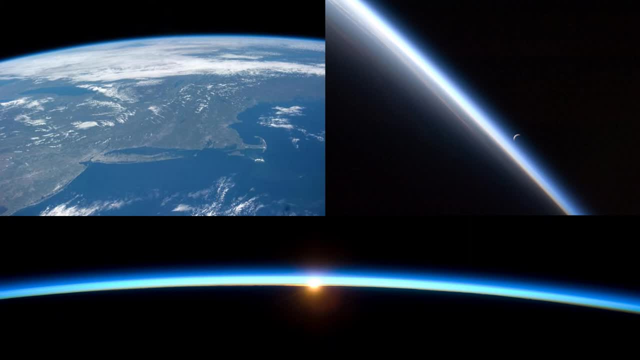 the apple than the atmosphere is to the Earth. You can also represent this error on a standard globe. So say you have a globe of an Earth in a school room. Well, the atmosphere would be about as thick as a dollar bill placed on the surface of an apple. So if you have 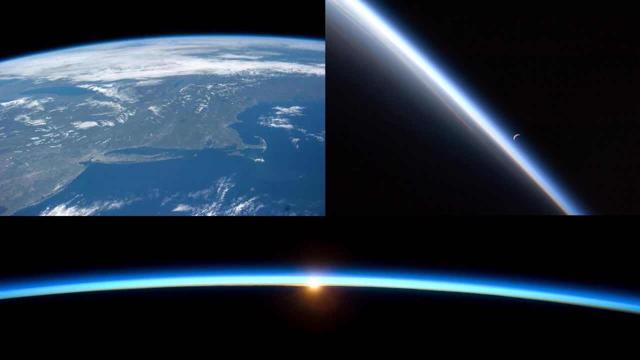 a globe like a standard, will you also be able to represent the entire, sooner and the future? That'll probably depend on how fragile the atmosphere is. The atmosphere is 20 times thicker than the skin of an apple, and in all months it's about 40 times thicker than. 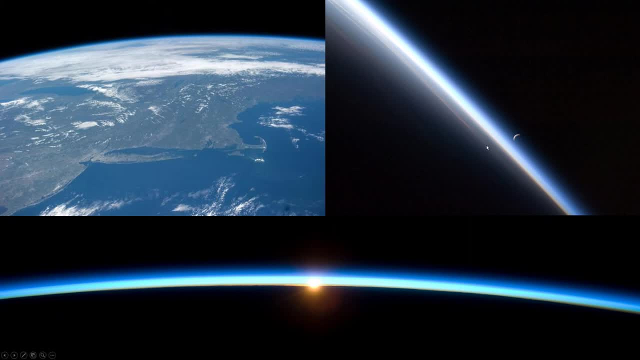 the skin of an apple. That's what these images show you, just to give you an idea of how thin the atmosphere is. So it does offer you a bit of perspective When we talk about global warming and climate change. it does give you perspective. 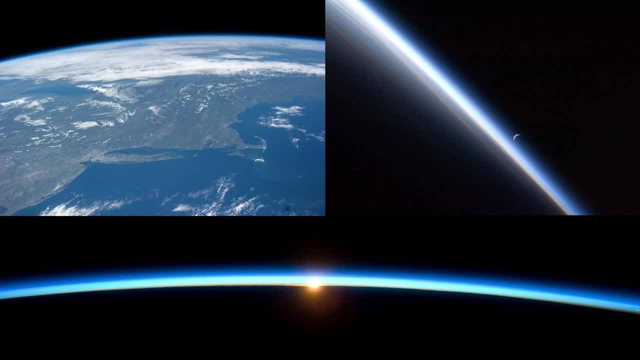 So what is Earth? allowing you to understand just how fragile it can be and how important it is to keep this thing going for us, because without it, as we'll learn soon, we'll start to see that we would not be here if it weren't for this atmosphere. 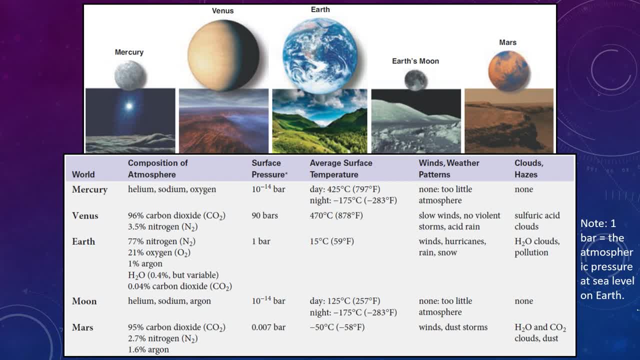 So the atmospheres of the terrestrial worlds are even more varied than their geologies. The figure here at the top shows global and surface views of each world. The table below lists general characteristics of the atmospheres. You'll notice vast differences between the worlds. 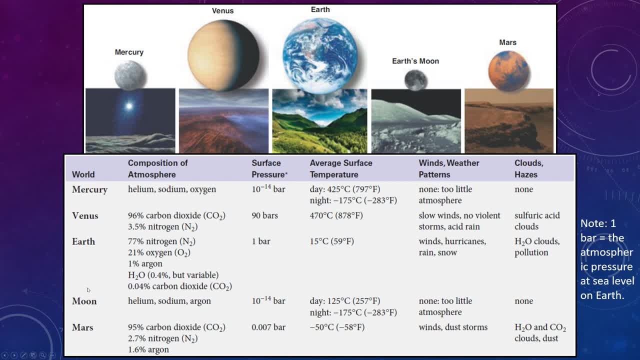 So take a look at the Moon and Mercury in this table. So Mercury's at the top, the Moon is down toward the bottom. The Moon and Mercury have such little atmosphere that it's reasonable to call them airless. They have no wind or weather of any kind. 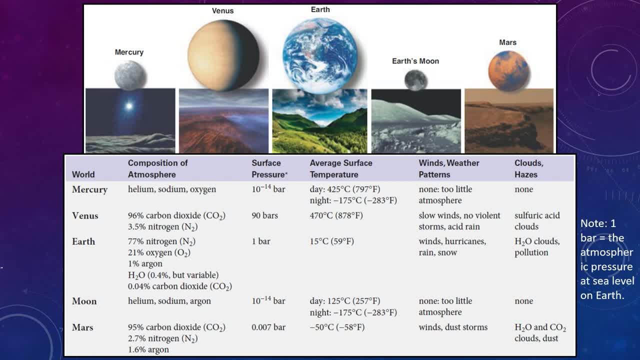 And at the other extreme, Venus is enshrouded by a thick atmosphere composed almost entirely of carbon dioxide, giving it conditions so hot and harsh that not even robotic space probes can survive there for long. Mars, which is at the bottom of the table, also has a carbon dioxide atmosphere. 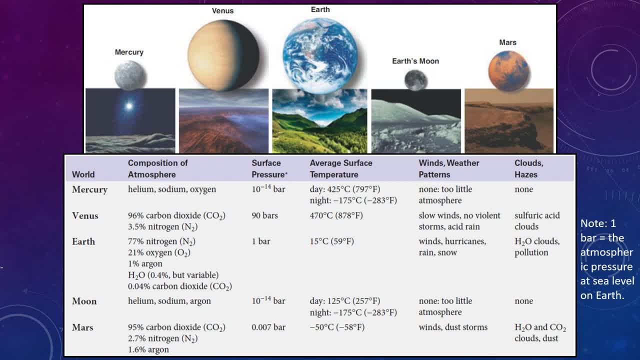 but its air is so thin that your body tissue would bulge painfully if you stood on the surface without a pressurized spacesuit. Only Earth has just right conditions that allow liquid water on the surface, making it hospitable to life. So this is again one of those really useful reference slides. 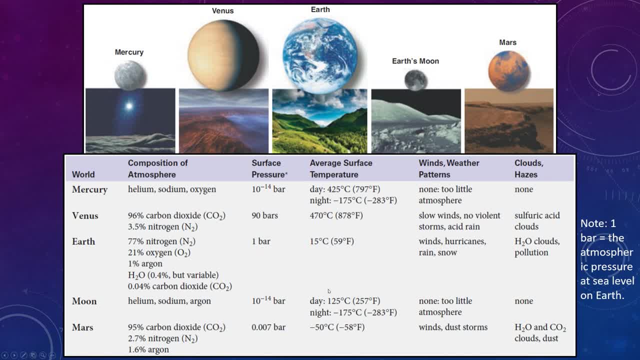 I won't go through everything, but it gives you the composition, pressure, average surface temperature and so on for each of the different planets And it really allows you to see how important different aspects of them become. So we'll especially be talking about greenhouse gases in this lecture toward the end. 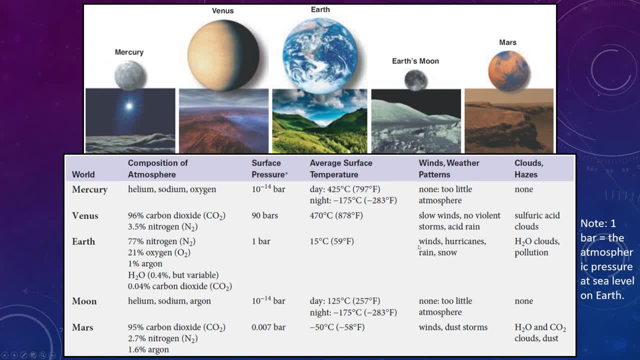 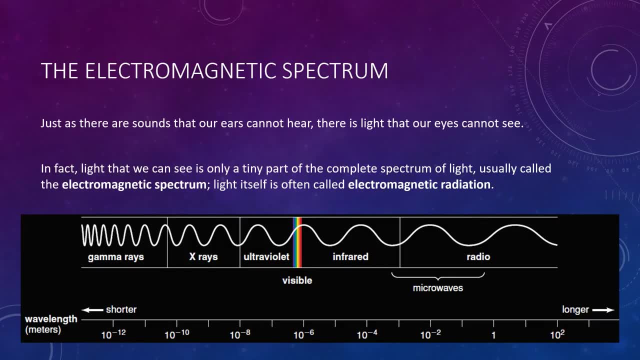 and we'll refer back to this average surface temperature pretty soon. So if you ever need this slide, it's a great one to reference. but let's dig into this a little bit more deeply Now. this is actually a slide from a future lecture on light. 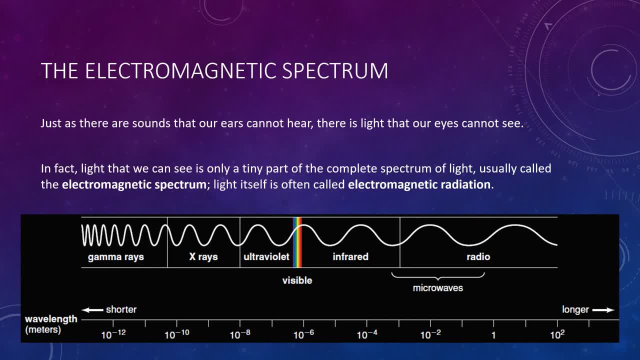 but I figured just throwing this single slide into this lecture now is pretty useful. So you can hear me say lots of different terms relating to light. We, as humans, we see visible light, So we see this tiny little fraction here, But there are more kinds of light that we can't see. 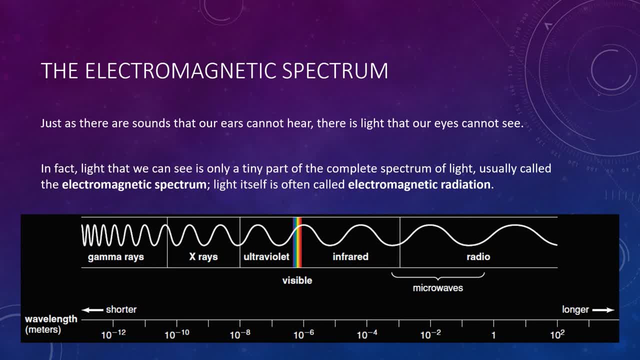 just like we have other sounds that we can't hear. Think of maybe a dog whistle. Well, there's lots of other types of light. We see visible, Some animals see in infrared, But there also exists Micro and radio waves. And then towards the more energetic side of things. 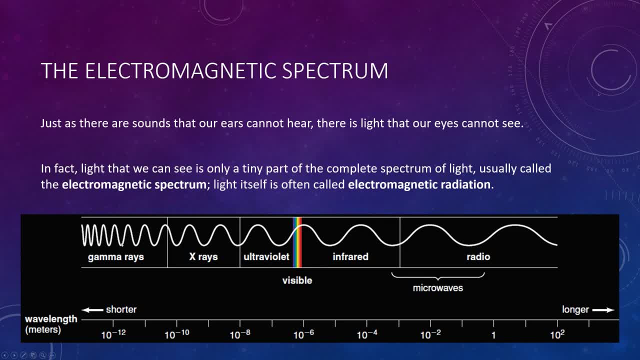 we have ultraviolet X-rays and the most energetic type of lights called gamma rays. So there isn't a lot of purpose to the slide here yet, But again you're going to hear me say a couple of these different types of light. 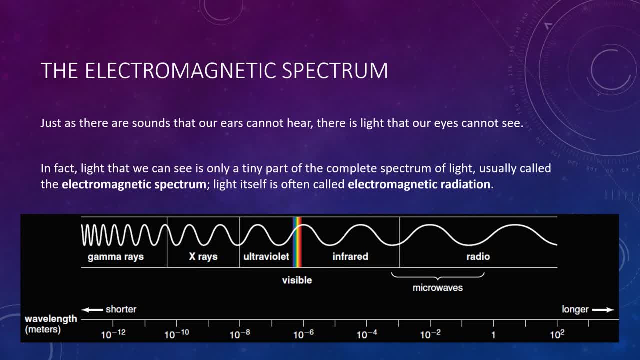 throughout the next several lectures, So I figured I'd throw it in, just so you know where it's coming from. Together, all of these different types of lights make up what we call the electromagnetic spectrum, which is just, you know, the electromagnetic spectrum. 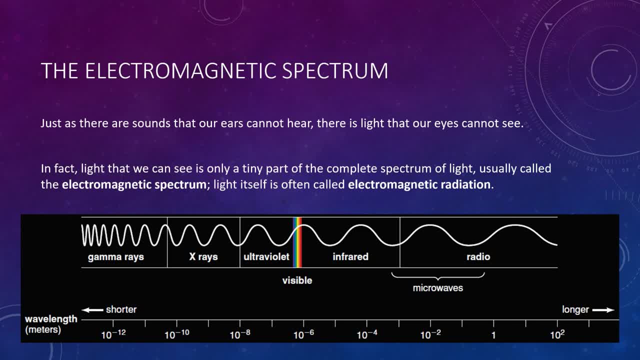 So you can see the electromagnetic spectrum. It's a spectrum in which all light exists, So light itself is technically radiation, And so we call it electromagnetic radiation, where it gets that name, because it's made up of both electric and magnetic waves, Things we'll learn about in the future. 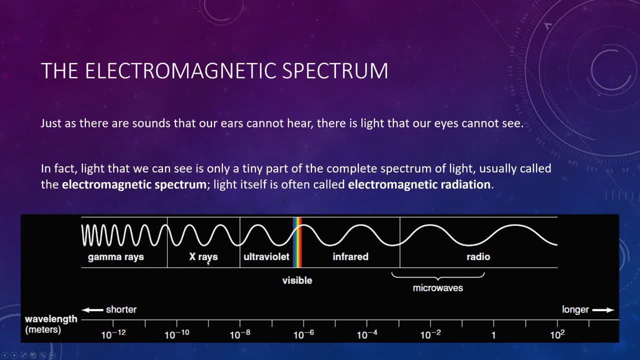 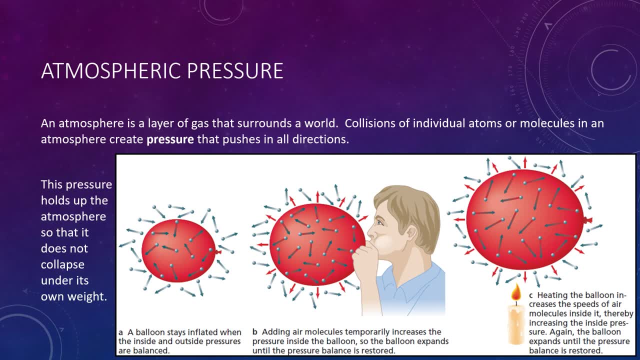 The point is, you just need to know that if you hear gamma, X-ray, whatever, it's just another type of light, All right. So an atmosphere is a layer of gas that surrounds a world. Collisions of individual atoms or molecules in an atmosphere. 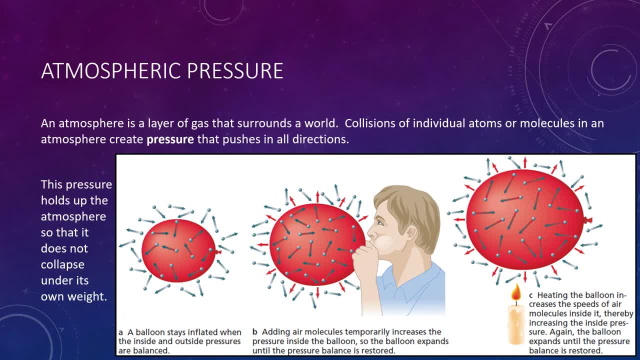 creates a pressure that pushes in all directions On Earth. for example, the nitrogen and oxygen molecules in the air fly around in an average speed of about 500 meters per second, which is actually fast enough to cross your bedroom 100 times in a second. 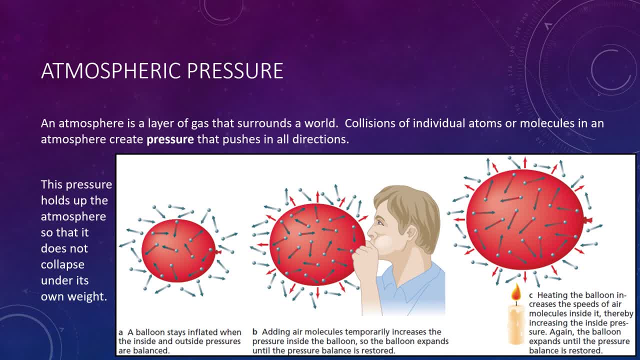 Given that a single breath of air contains more than a billion trillion molecules, you can imagine just how frequently molecules collide. On average, each molecule in the air around you will suffer about a million collisions in the time that it takes me to explain this. 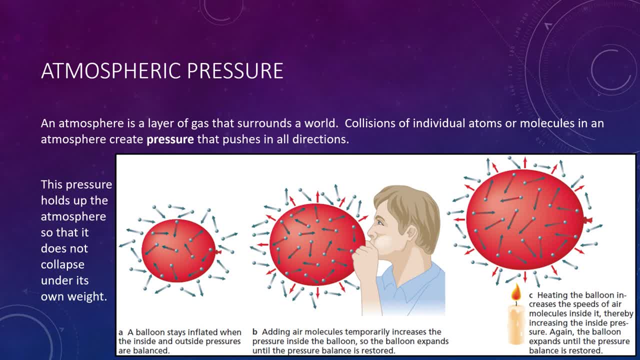 These collisions create pressure that push in all directions, and this pressure holds up the atmosphere so that it does not collapse under its own weight. A balloon offers a good example of how pressure works in a gas. The air molecules inside a balloon exert pressure. 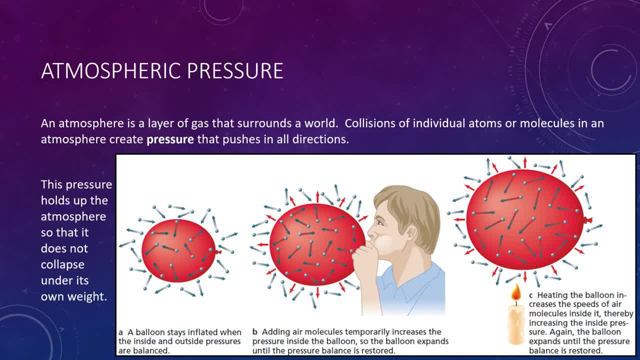 pushing outward as they constantly collide with the air. However, at the same time, outside air molecules collide with the balloon's outer surface, exerting pressure that by itself would make the balloon collapse. A balloon stays inflated when the inward and outward pressure are balanced. 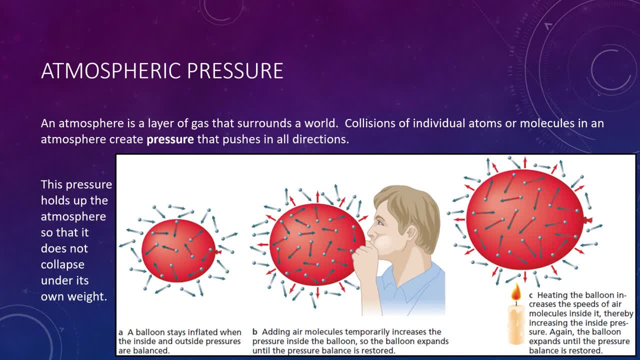 Imagine that you blow more air into the balloon. now The extra molecules inside means more collisions with the balloon wall, momentarily making the pressure inside greater than the pressure outside. The balloon therefore expands until the inward and outward pressure are again in balance. If you heat the balloon, the gas molecules begin moving faster. 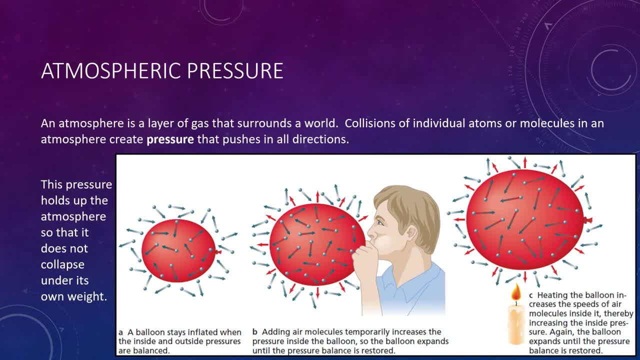 and collide harder and more frequently with the inside surface, which also momentarily increases the inside pressure, until the balloon expands. As it expands, the pressure inside it decreases and the balloon comes back into pressure balance. Conversely, cooling a balloon will make it contract. 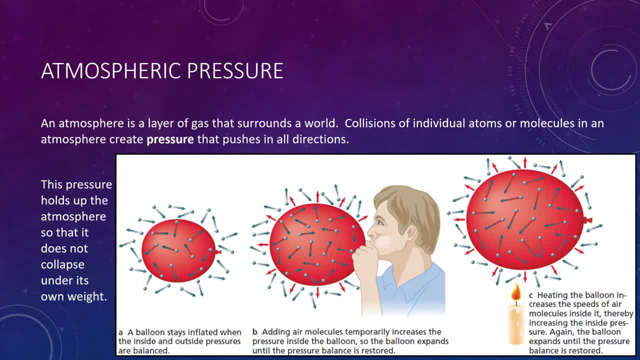 because the outside pressure would then momentarily exceed the inside pressure. So it's not a, it's a great comparison really. I mean comparing the Earth's atmosphere to a balloon. So again, adding more molecules or heating the balloon causes it to expand. 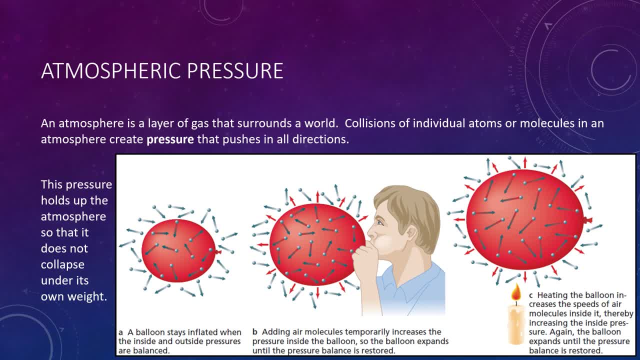 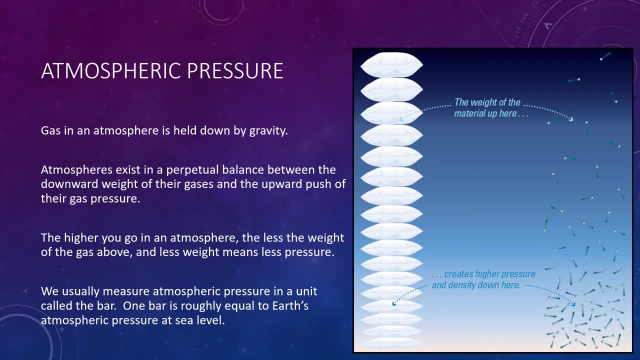 because of this difference in pressure, And this is a great analogy when we compare to the Earth's atmosphere or any atmosphere. So we can understand atmospheric pressure by applying similar principles. Gas in an atmosphere is held down by gravity. The atmosphere above any given altitude therefore has some weight that presses downward. 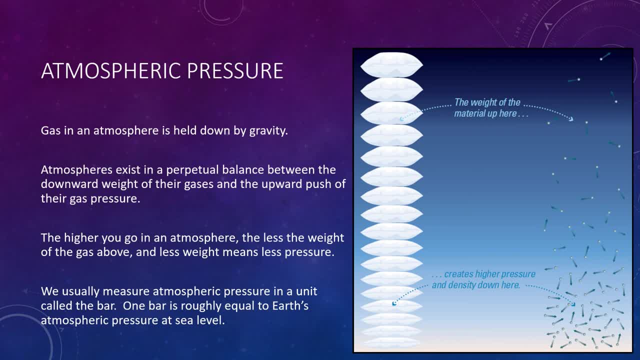 tending to compress the atmosphere beneath it. At the same time, the fast-moving molecules exert pressure in all directions, including upward, which tends to make the atmosphere expand. So planetary atmospheres exist in a perpetual balance between the downward weight of the atmosphere and the downward weight of the atmosphere. 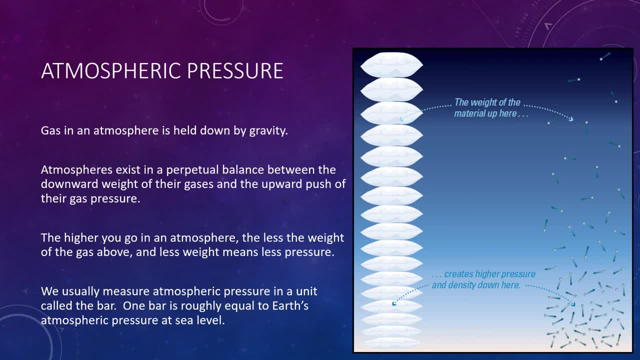 The atmosphere is the downward weight of their gases and the upward push of their gas pressure. The higher you go in an atmosphere, the less the weight of the gas above you and thus the less weight means less pressure. That is why the pressure decreases as you climb a mountain or ascend in an airplane. 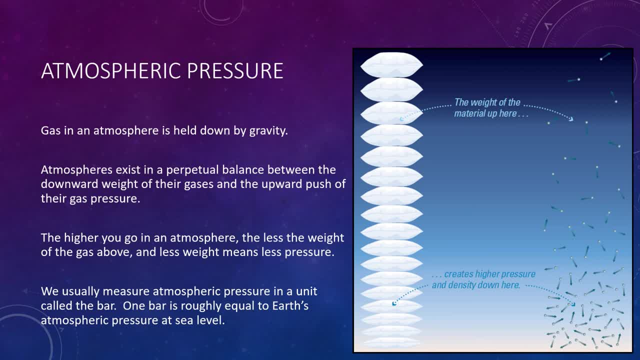 You can visualize this concept by imagining an atmosphere as a very big stack of pillows. like you see in the figure here on the right, The pillows at the bottom are highly compressed because of the weight of the pillow. In other words, going upward, the pillows are less and less compressed because of the weight that lies on top of them. 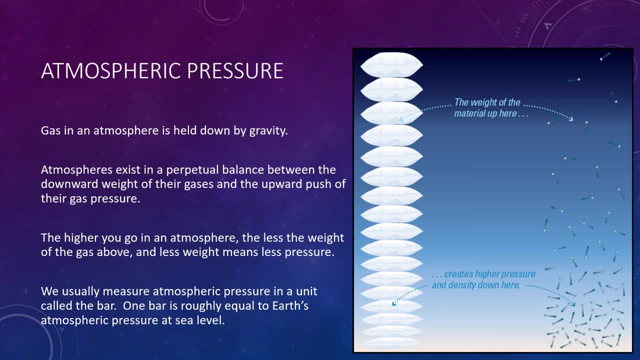 In planetary science we usually measure atmospheric pressure in units called a bar, which is like as if it was a barometer. One bar is roughly equal to the earth's atmospheric pressure at sea level. It is also equivalent in terms of numbers to 1.03 kilograms per square centimeter. 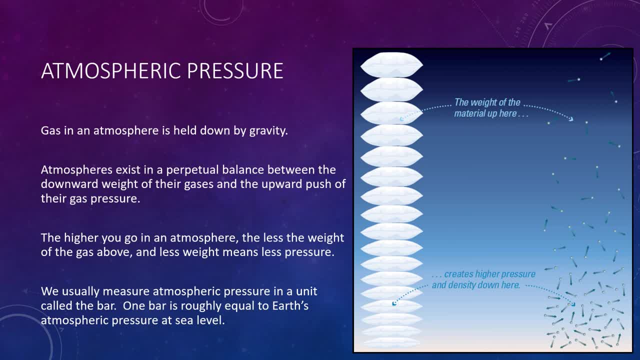 which is roughly equal to the earth's atmospheric pressure at sea level. The barometer is roughly equal to the earth's atmospheric pressure at sea level. The barometer is roughly equal to the earth's atmospheric pressure at sea level. The barometer is roughly equal to the earth's atmospheric pressure at sea level. 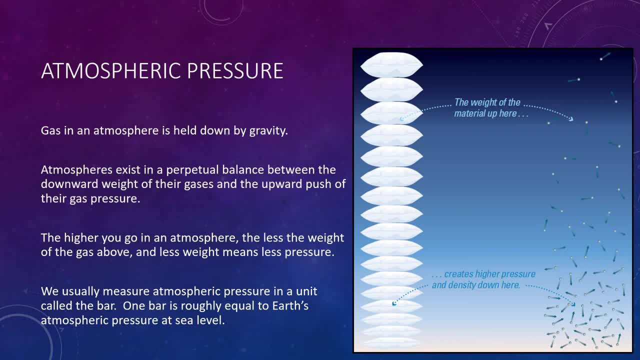 In other words, if you gathered up all the air directly above any one square inch of earth's surface, you would find that it weighed, on average, about 14.7 pounds. Now that might make you wonder why you don't feel the earth's atmospheric weight bearing down on you. 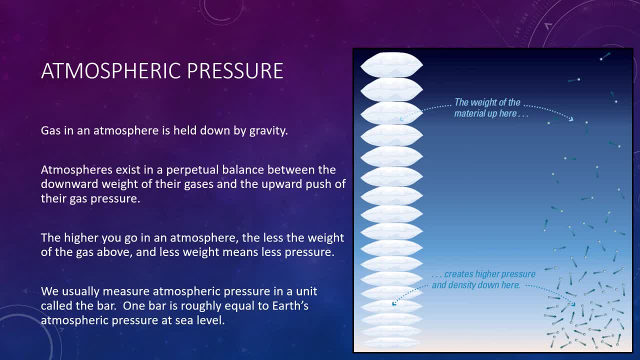 After all, if we placed 14.7 pounds of weight on every square inch of your shoulders, you'd certainly feel that downward pressure, But you don't feel the atmospheric pressure on your shoulders. But you don't notice the atmospheric pressure for two reasons. 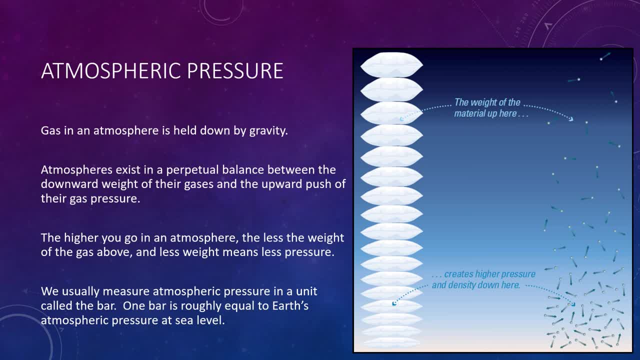 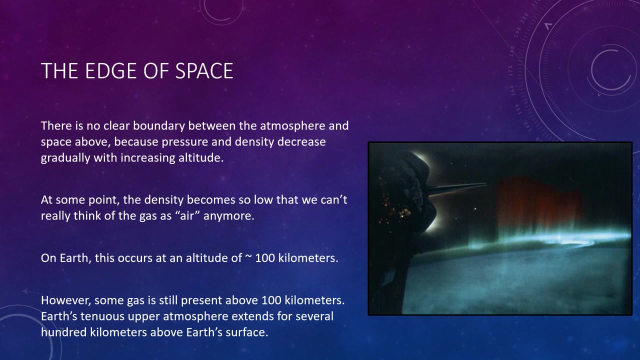 First, the pressure pushes in all directions, so it pushes upward on you as well as downward. Second, the fluids in your body push outward with an equivalent pressure, so there is no net pressure trying to compress or expand your body. If you studied the previous figure, you'd see that there is no clear boundary between atmosphere and the space above. 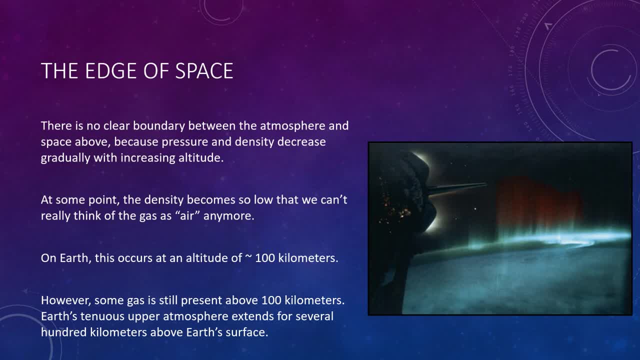 because pressure and density decrease gradually with an increasing altitude. At some point the density becomes so low that we can't really think of the gas as air anymore. Collisions between atoms or molecules are rare at these altitudes and the gas is so thin that it would look and feel as if you had already entered space. 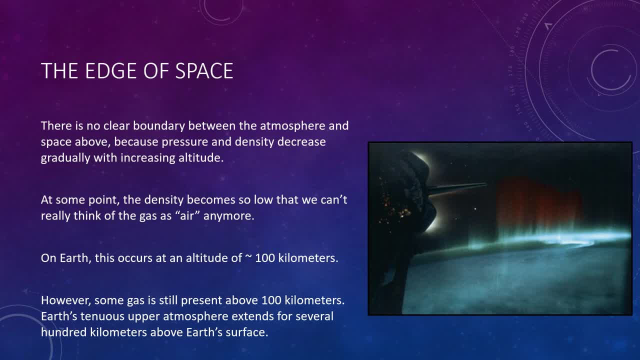 On Earth. this occurs at an altitude of about 100 kilometers. Above that, the sky is black even in the daytime, much like the sky on the moon. The altitude is often described as the edge of space. However, some gas is still present above this 100-kilometer mark. 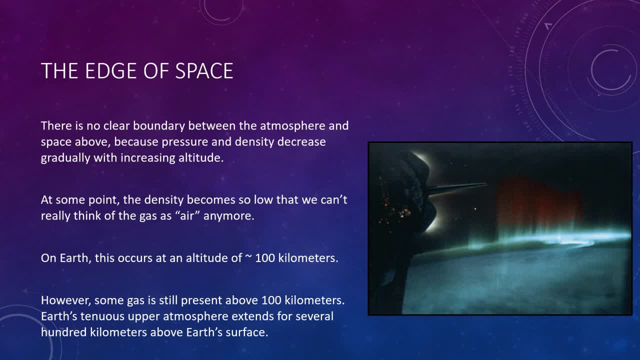 Earth's tenuous upper atmosphere extends for several hundred kilometers above the surface. The space station and many satellites orbit Earth within these outer reaches of the atmosphere. The low-density gas may be barely noticeable under most conditions, but it does still exert drag on orbiting spacecraft. 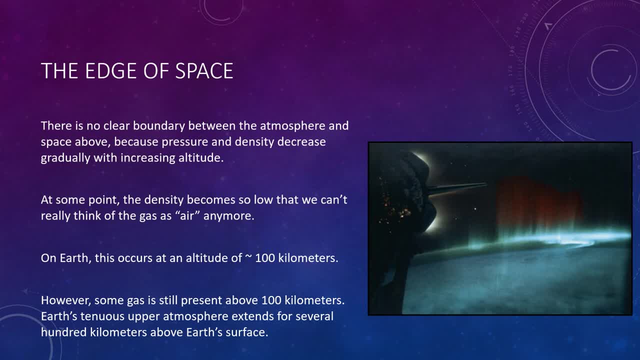 That is why satellites in low-Earth orbit are able to spiral downward, eventually burning up as they re-enter denser layers of the atmosphere. So here on the right, you see a figure. We have proof of this low-density gas extending into what we often think of as space. 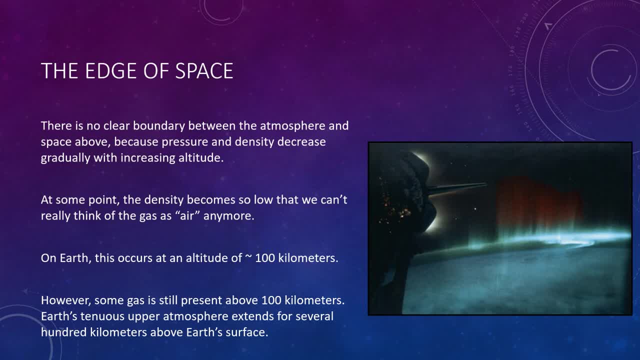 as you can see from the visible glow of the gas around the space shuttle's tail in this photograph. So you can see that gas glowing right here. So there is gas out there, but it also shows the aurora in the background created by interactions between charged particles and the atmospheric gases. 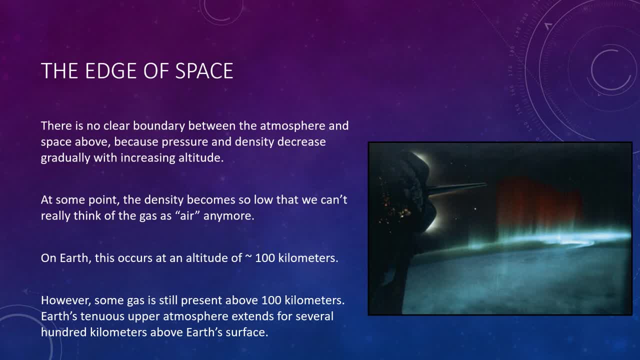 at altitudes above 100 kilometers, well below the shuttle. So most of Earth's gases lie below 10 kilometers, but that does not mean that there is nothing above that, So you can still see proof of gases being above this, even though it's dark out. 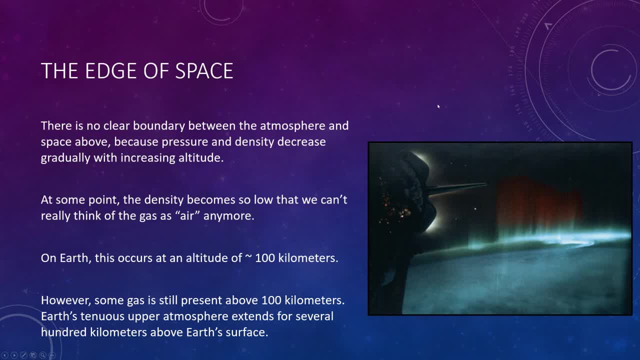 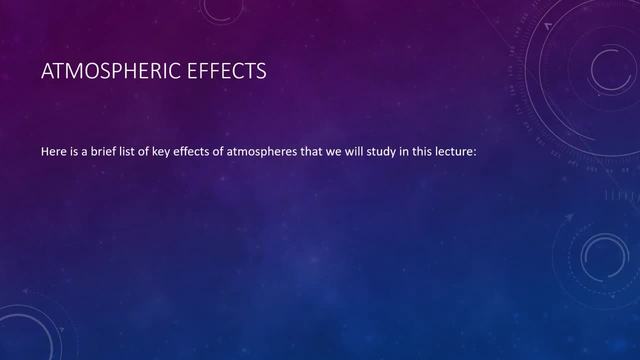 even in the daytime, because there's no gases for the light to scatter off. of More things that we'll learn about soon. Alright, so Earth's atmosphere is obviously important for our existence, but the full range of atmospheric effects is greater than most people realize. 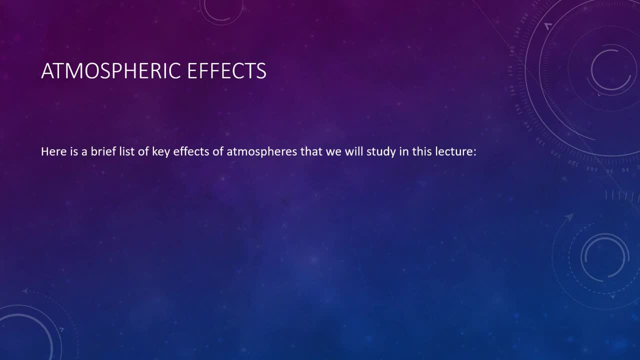 To provide context for our study of planetary atmospheres, here's a brief list of key effects of planetary atmospheres that we will study throughout these lectures. As we've seen, atmospheres create pressure that determines whether liquid water can exist on the surface. 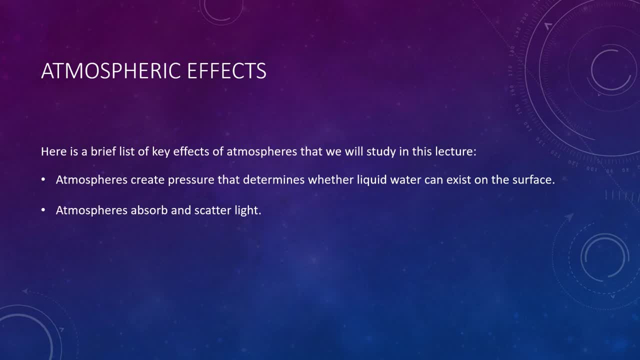 Atmospheres also create pressure that determines whether liquid water can exist on the surface. Atmospheres also absorb and scatter light. Scattering can make daytime skies bright and absorption can prevent dangerous radiation from reaching the ground. Atmospheres can create wind and weather. 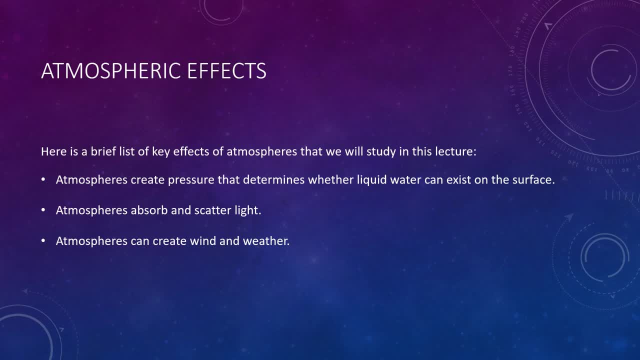 and play a major role in long-term climate change. Interactions between atmospheric gases and the solar wind can create a protective magnetosphere around planets with strong magnetic fields, something we'll talk about in our next lecture Also. Also also, we can make planetary surfaces warmer than they would be otherwise via the Greenhouse Effect. 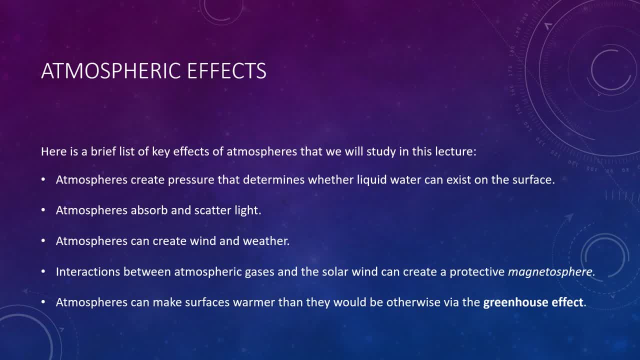 Now, this greenhouse effect is arguably the most important effect that an atmosphere can have on its planet, and so we will therefore focus our attention on this first. So you've probably heard of the greenhouse gas or, I'm sorry, of the greenhouse effect. 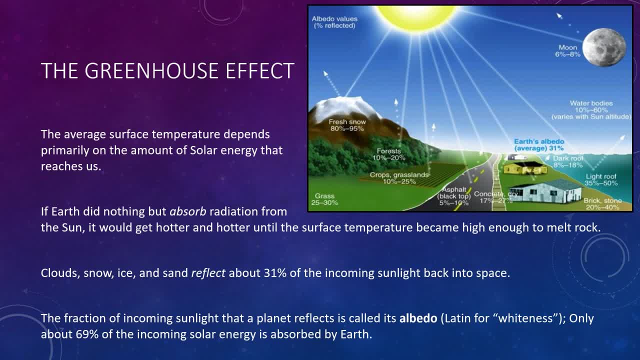 because it is an important part of the environmental problem known as global warming or climate change. Well surprised to learn that the greenhouse effect is also crucial in the existence of life on Earth. Without this greenhouse effect, Earth's surface would have been too cold for liquid. 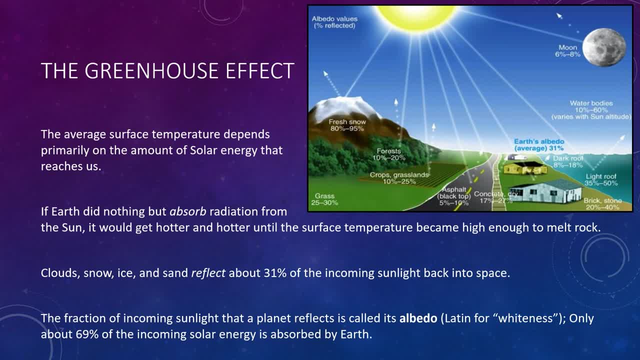 water to flow and for life to flourish. So let's explore the greenhouse effect and how it can warm planetary surfaces. Well, very little heat, as we've already learned, comes from inside of our planet, So the average surface temperature of the Earth depends almost. 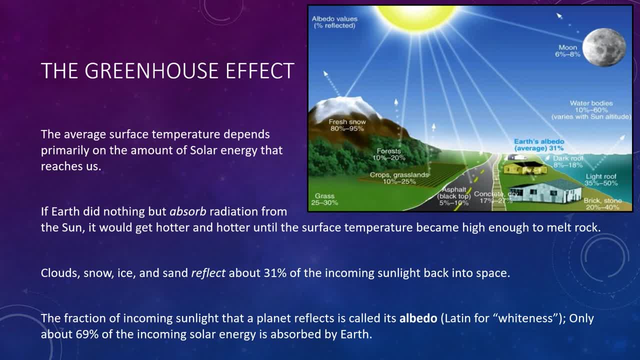 entirely on the amount of energy that reaches us from the sun. If Earth did nothing but absorb radiation from the sun, well, it would just get hotter and hotter until the surface temperature became hot enough to melt rock. Happily, that does not happen. One reason: 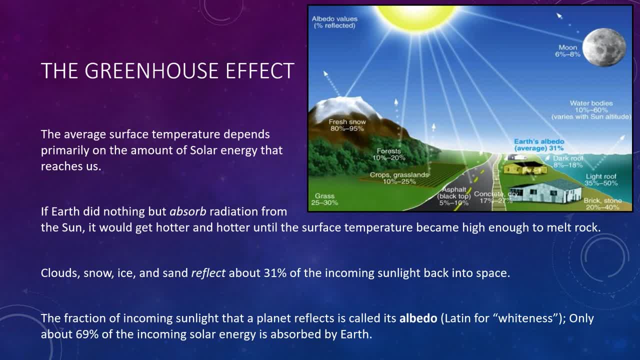 for this is that the clouds, snow, ice and sand and many other surface features reflect, on average, about 31% of the incoming sunlight back into space. The fraction of incoming sunlight that comes back into space is the fraction of the incoming sunlight that comes. 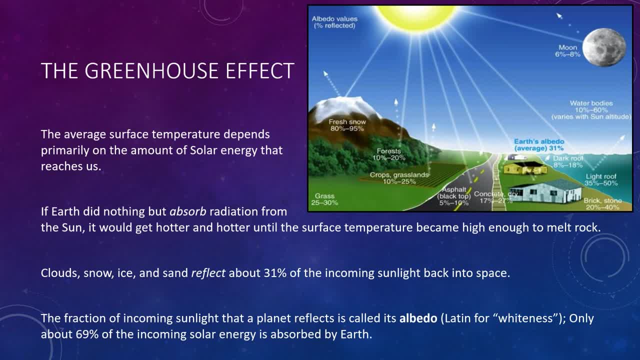 back into space. The fraction of incoming sunlight that comes back into space is: the fraction of the incoming sunlight that comes back into space, The fraction of incoming 晚上 on the planet reflects is called its albedo, which is Latin for whiteness Only. 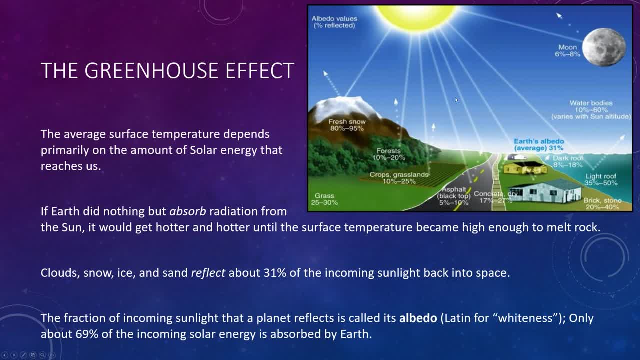 about 69% of incoming solar energy there is absorbed by the Earth. So that's what this image here is trying to show you. in the top right, It's just showing you various surfaces and how much of the energy from the sun is being reflected. So you'll 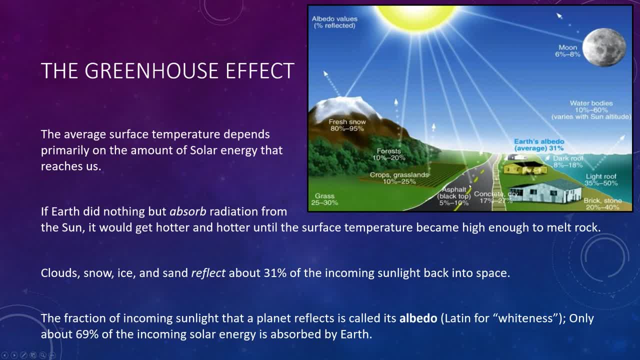 notice something like fresh snowpack If you have new snow on the ground. well, it will. However, if you step onto an asphalt road, a blacktop road, it's only reflecting about 5 to 10 percent. The rest is being absorbed. 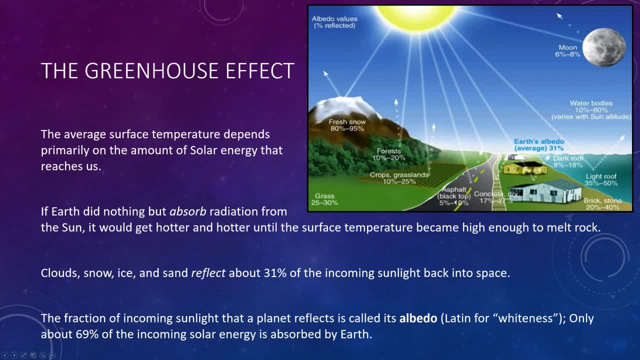 So this is why, for example, it feels so much warmer on an asphalt road or, for example, maybe if you're wearing a black shirt versus a white shirt. in the summer heat, A black shirt will make you feel a lot warmer because it is more effective at absorbing. 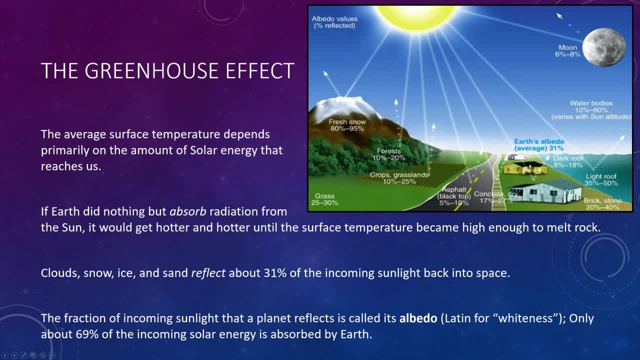 the sun's energy. So this is actually why rooftops now are becoming lighter, For example. you want a lighter roof so that a lot of the sun's energy is reflected off and you have less of a heating bill to worry about, And also you can notice that the moon does actually reflect some of the solar energy. 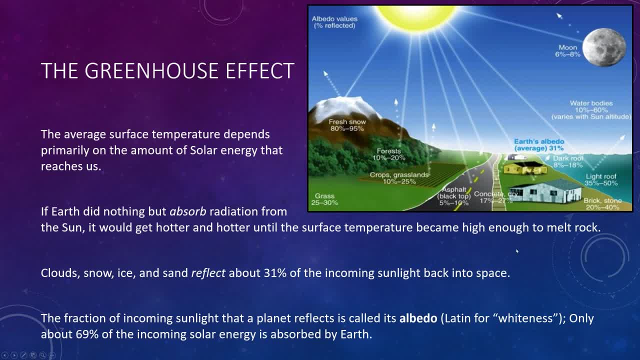 This is why we see the moon. It reflects some light that we then see on Earth. So if it didn't do that, it would just be black and we would never really see it. So this is very important. So we're starting to understand already just how important this greenhouse effect can be. 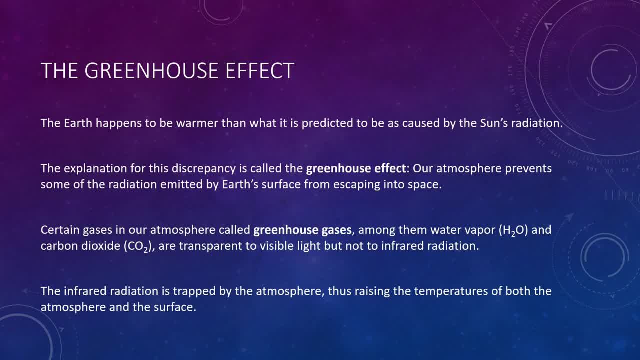 So let's continue our discussion on this. Well, it turns out that we now know that Earth happens to be warmer than what is predicted to be caused just by the sun's radiation alone. The explanation for this discrepancy is called the greenhouse effect. Our atmosphere prevents some of the radiation emitted by Earth's surface from escaping. 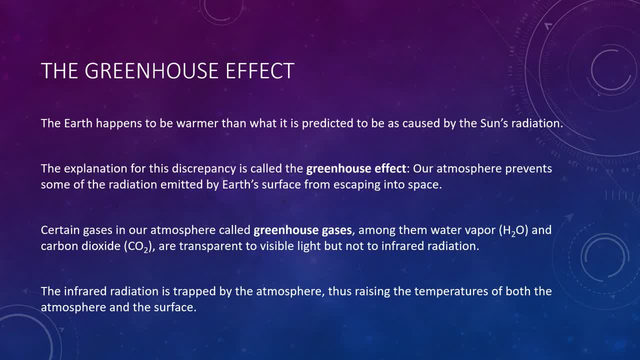 into space. Certain gases in our atmosphere, called greenhouse gases among them, including water vapor and carbon dioxide, are transparent to visible light, but not to infrared light. So what that means is visible light has no trouble entering our atmosphere and warming the surface. 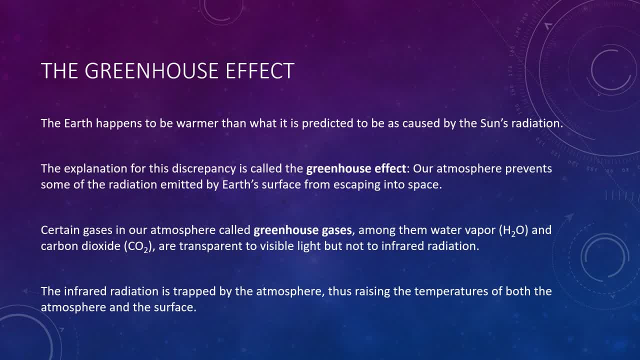 But once our surface is warmed, that infrared radiation that is emitted coming from the heated surface is partially trapped by the atmosphere now, thus raising the temperature of both the atmosphere and the surface. So visible light from the sun has no problem getting through to the surface, but once it 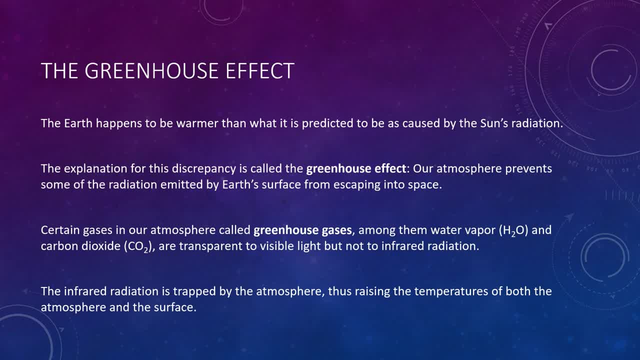 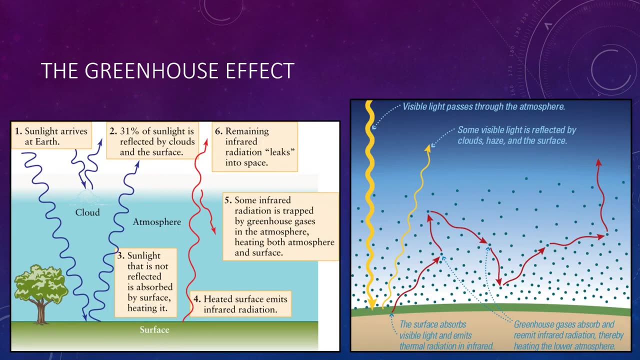 hits the surface, the surface will emit infrared radiation and that gets trapped by the greenhouse gases. So we can start to see why that is a little important, and we'll elaborate on that as we continue. The net result is that greenhouse gases tend to slow the escape of infrared radiation from 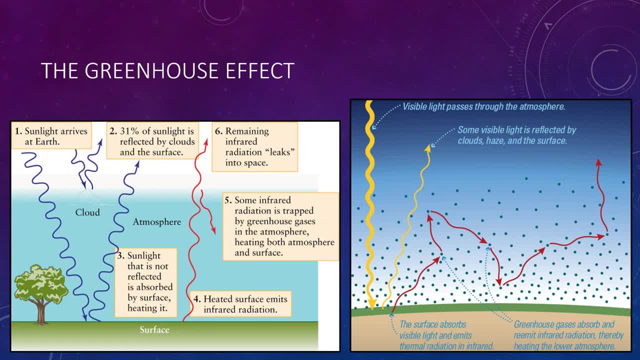 the lower atmosphere, while their molecular motions heat the surrounding air. In this way, the greenhouse effect makes the surface and the lower atmosphere warm. In this way, the greenhouse effect makes the surface and the lower atmosphere warm. So let's continue our discussion on this. 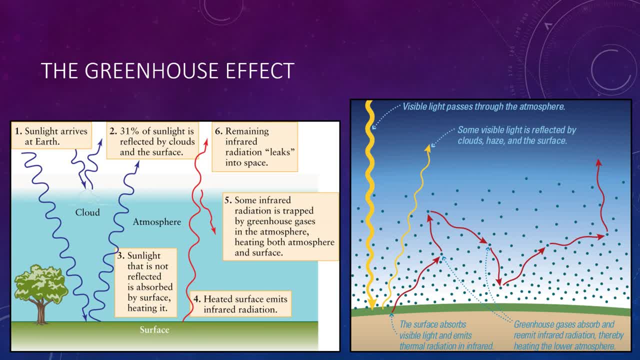 warmer than they would be from sunlight alone. The more greenhouse gases present, the greater the degree of surface warming. All the energy trapped by the greenhouse effect still does escape into space, but just not as directly as it would have otherwise. A blanket offers a great analogy. 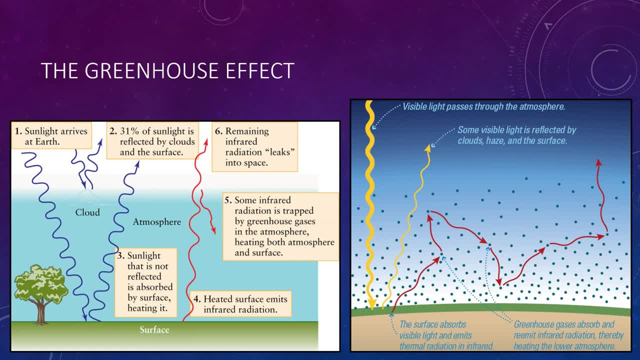 You stay warmer under a blanket, not because the blanket itself is providing any heat, but because it slows the escape of your body heat into the cold outside air. The warming caused by the greenhouse effect gives our planet the moderate temperatures needed for the existence for life. 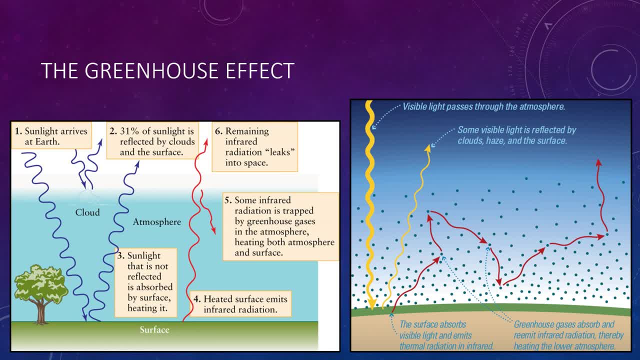 For more than a century, however, our technological civilizations have been adding greenhouse gases to the atmosphere at an unprecedented rate. So, basically, we are adding layers to our blanket right. So imagine laying in bed: it starts to get a little warm, but you keep adding more blankets. 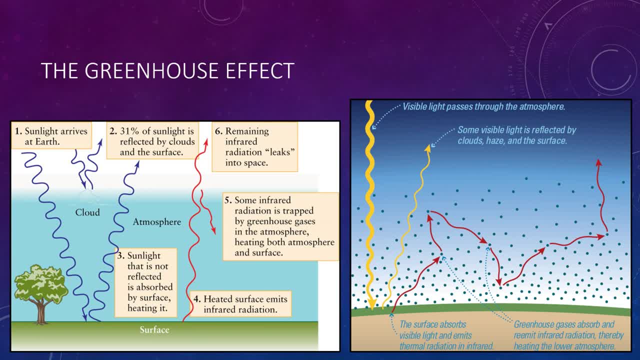 on top of you. Well, you're going to get more and more warm. So that's effectively what is happening here. We're adding our Earth's blanket by all of our technological advances in producing CO2 and outputting that into the atmosphere. 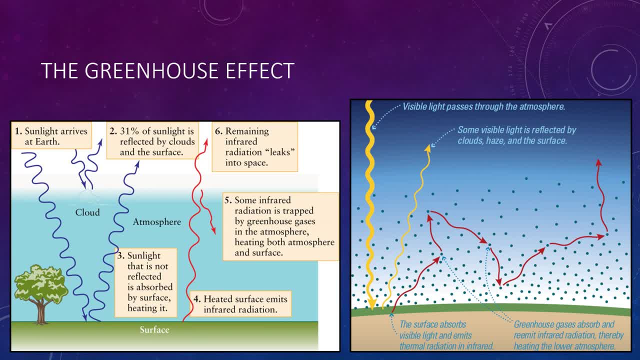 So we're adding blankets to the surface. So we do have an effect that we'll talk about in a future video, But the point is right now at least to understand this greenhouse effect. So these two images show the exact same thing. I just figured it'd be useful to see two perspectives. 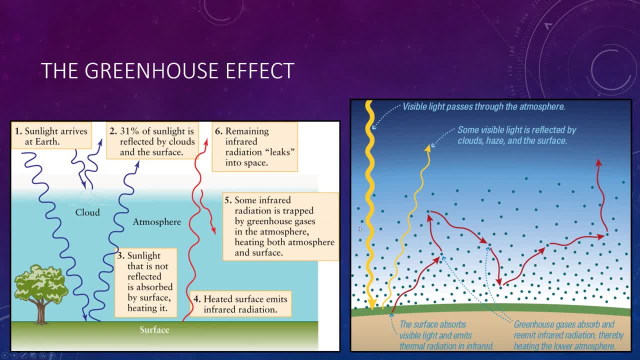 of it. But the idea is is that visible light from the sun passes through the atmosphere. It then strikes the earth. Some of it is reflected. about 31% of it is reflected away from the earth right back into space, But nearly 70% is absorbed on average. 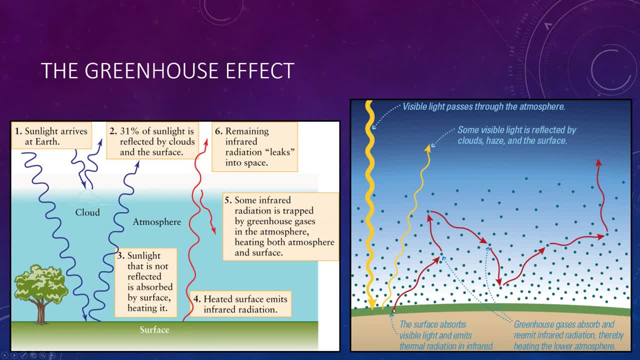 Well, once it absorbs the energy, that can be remitted. but as infrared radiation and greenhouse gases are very good at blocking that infrared radiation, So it takes much longer. It takes much longer. So it takes much longer for this infrared radiation to escape. 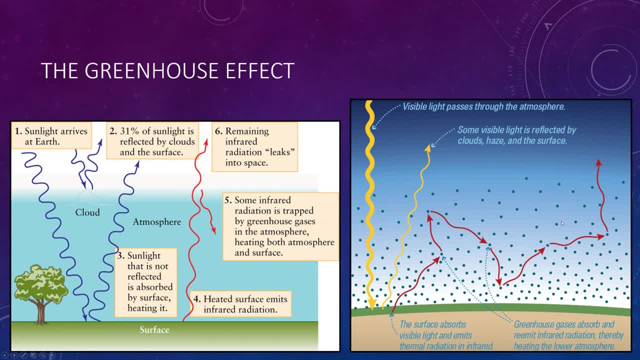 So as we keep building blankets, we're keeping this warmth in for more and more time, And so the net effect is that it warms up. So we'll get back into this later on, when we talk about the human effect a little bit. 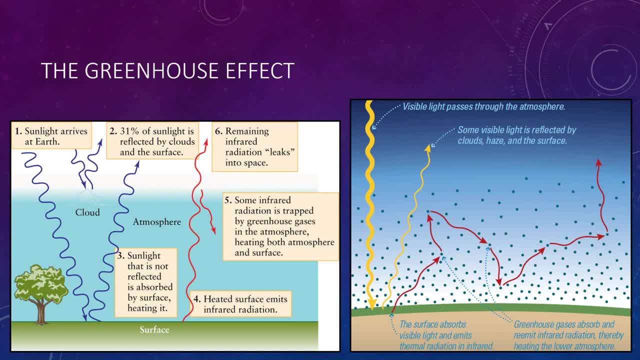 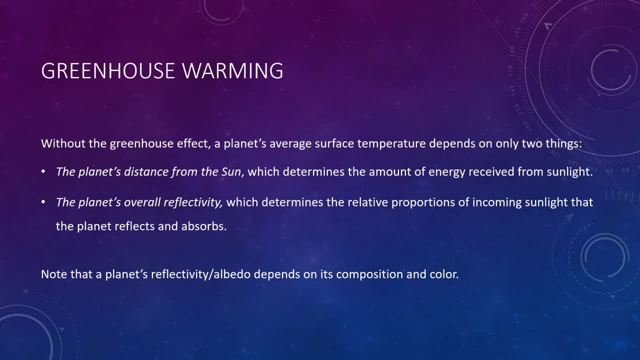 But just know that this is a big deal And hopefully you can kind of see that now with that greenhouse effect discussion we can better appreciate the importance of the greenhouse effect. So let's take a look at the greenhouse effect by comparing each planet's average surface. 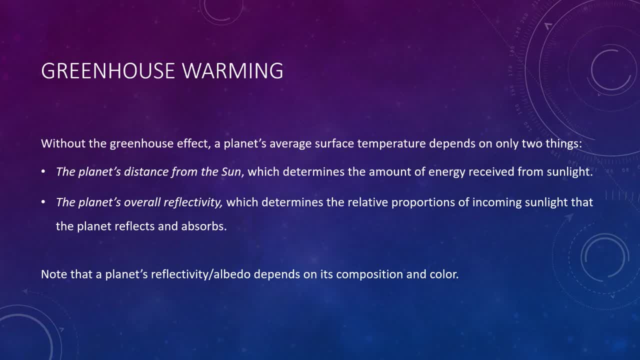 temperature or global average temperature, with and without it. Recall that a terrestrial planet's interior heat has very little effect on its surface temperature, so sunlight is the only significant energy source for the planet. Therefore, without the greenhouse effect, a planet's global average surface temperature. 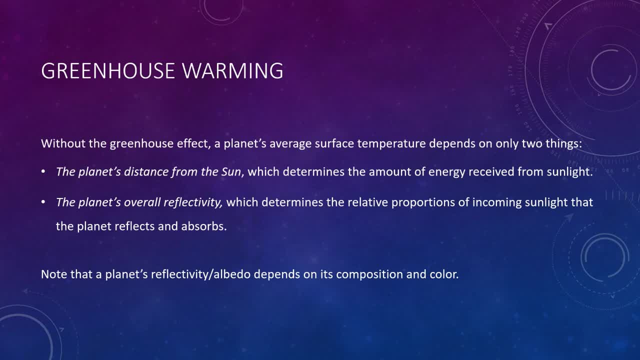 depends only on two things: The distance from the sun, which determines the amount of energy received from sunlight, and the distance from the sun, which determines the amount of energy received from sunlight, The closer a planet is. so this is a trend we've seen, but the closer a planet is to 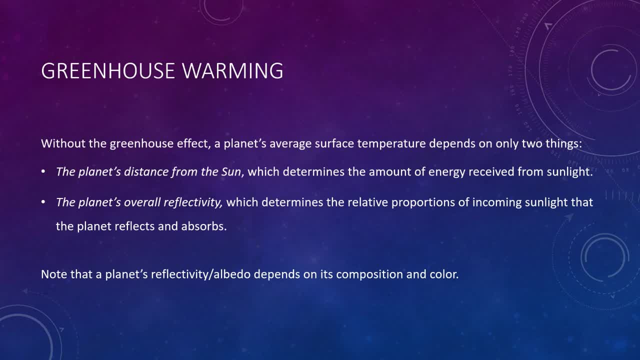 the sun, the greater the intensity of the incoming sunlight. The second is that the planet has an overall reflectivity and this determines the relative proportions of incoming sunlight that the planet reflects and absorbs. The higher the reflectivity, the less light absorbed and the cooler the planet. 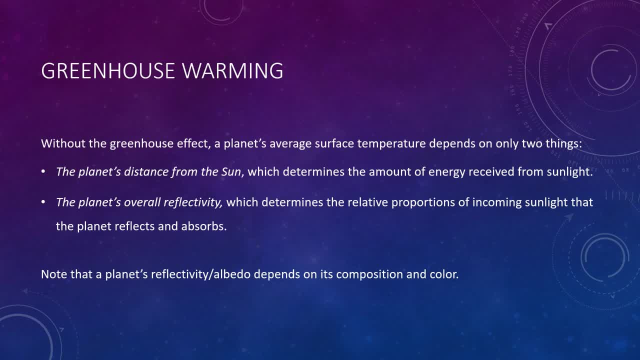 So note that the planet's reflectivity, or its albedo, depends on its composition and color. The colors reflect less light. So, for example, as we mentioned, snow and ice reflect about at least 70% of the light that hits them and absorb only 30%. 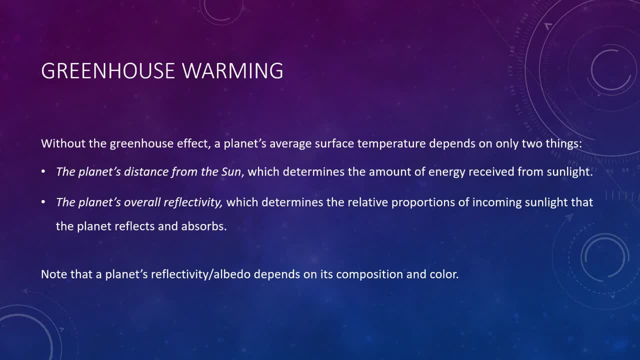 But things like rocks? they typically absorb about 80% of the energy and only reflect about 20%, So this is very important. So without the greenhouse effect, it only depends on distance and reflectivity. So let's take a look now at a table. 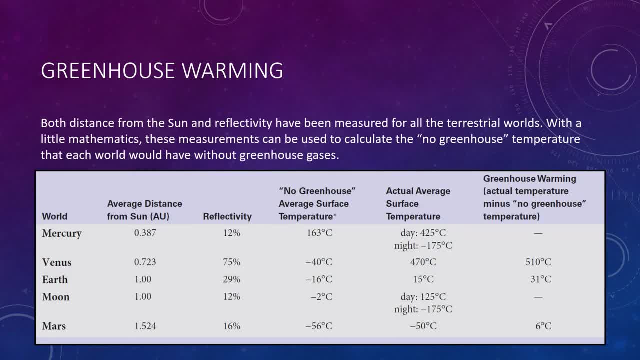 Showing what this looks like. Well, both distance from the sun and reflectivity have been measured for all of the terrestrial worlds. With a little bit of mathematics, these measurements can be used to calculate the quote. no greenhouse temperature that each world would experience without the greenhouse gas, without greenhouse. 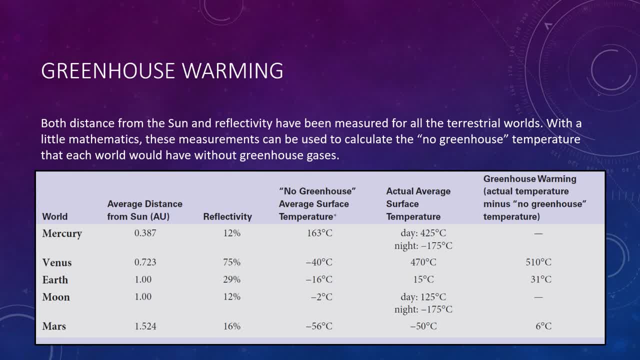 gases in their atmosphere. So this table shows the result. The no greenhouse temperature for Mercury and the Moon lie between their actual day and night temperatures. That's because they have little atmosphere and hence no greenhouse effect. So if you look at Mercury, the top one, and Moon, the second to last, they're…well let's. 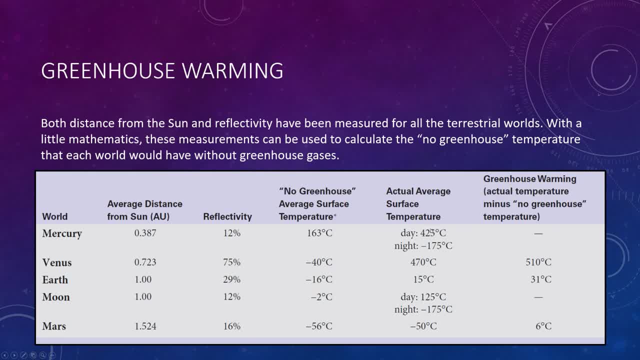 look at Mercury, Their day and night temperature ranges between negative 175 and 425 degrees Celsius. and if they had no greenhouse effect, well, their average surface temperature is right in the middle, And same for the Moon: It's right in the middle. 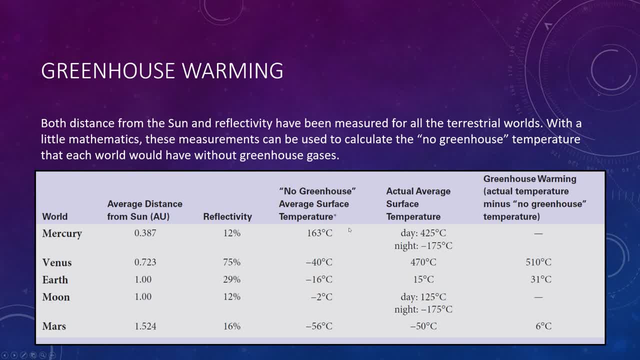 So because they don't have an atmosphere, well, they have no greenhouse effect, so their temperature won't really vary much without it. 3. Greenhouse effect: have a weak greenhouse effect. So Mars is the bottom one here, So that makes its global average. 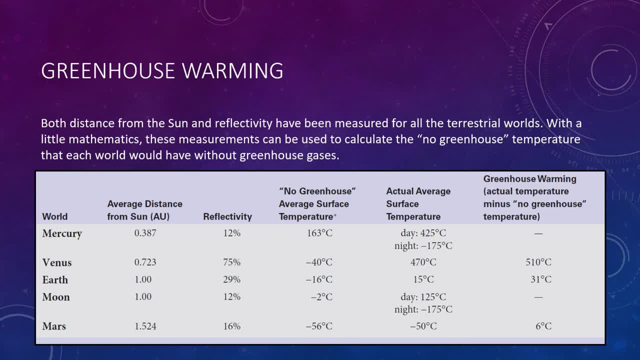 temperature about six degrees higher than it is with a no greenhouse temperature. right. So Mars is a little bit cooler than it would be otherwise, because it does have a thin atmosphere made out of mostly carbon dioxide. that does keep it a little bit warmer than it would be otherwise. 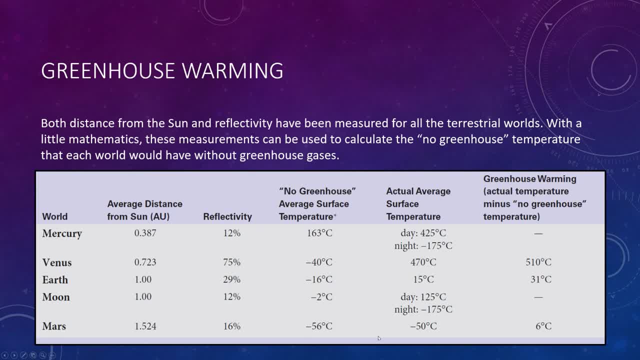 excuse me. So you can see the slight effect that that has. But Venus is the extreme case, with a greenhouse effect that bakes its surface to a temperature of more than 500 degrees Celsius at times, which is hotter than it would be otherwise. So we can see why the greenhouse. 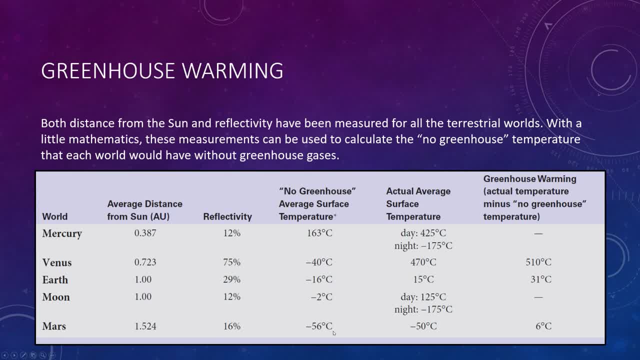 effect is so important on earth too because of this right. I mean, look at what happens. You have the thick atmosphere on Venus, Venus, and because of all those greenhouse gases in its atmosphere, it is nearly 500 degrees warmer than it would be otherwise. It'd be sitting at a cold minus 40 degrees Celsius without all 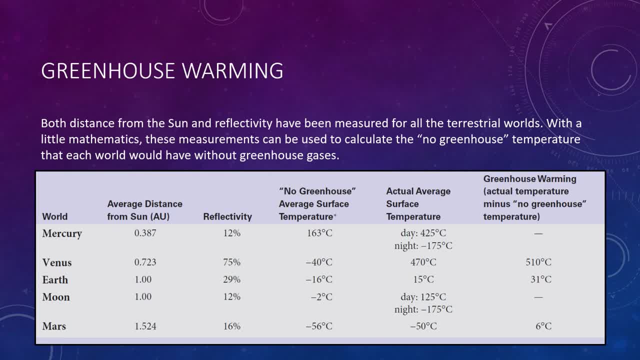 that greenhouse gas. So this is really important. So we can also see why it's important to life on Earth. now We've seen some of the extremes. Without the greenhouse effect, our planet's global average temperature would be about three degrees Fahrenheit, well below the freezing point. 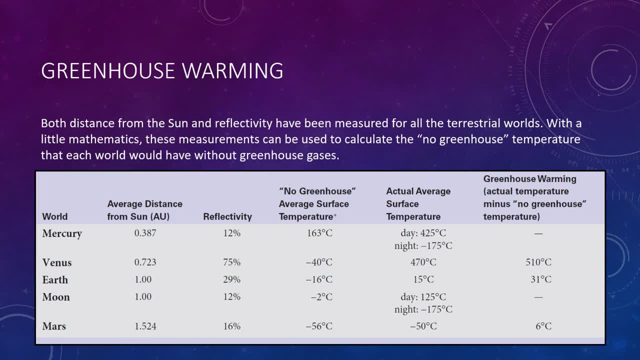 of water With it. the global average temperature today is about 59 degrees Fahrenheit, So that's about 31 degrees Celsius warmer than the no greenhouse temperature. So this is very important again, because if we keep adding layers of blankets to our atmosphere with our greenhouse gas, 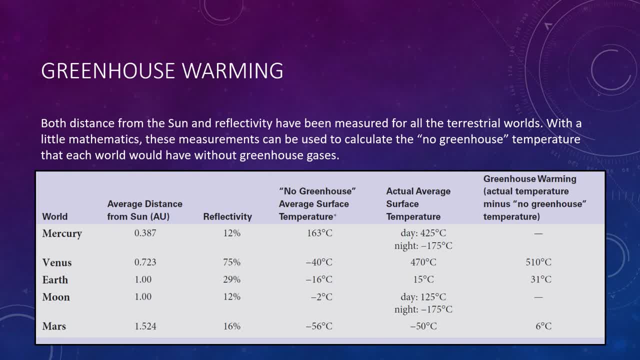 emissions, we are going to continually warm our surface. Just look at what happens to Venus when you have that much in the atmosphere. So I keep hitting at this. We will discuss the human influence of greenhouse gas emissions in the next episode And a couple lectures from now. we'll talk a little bit about climate change and stuff like that, But 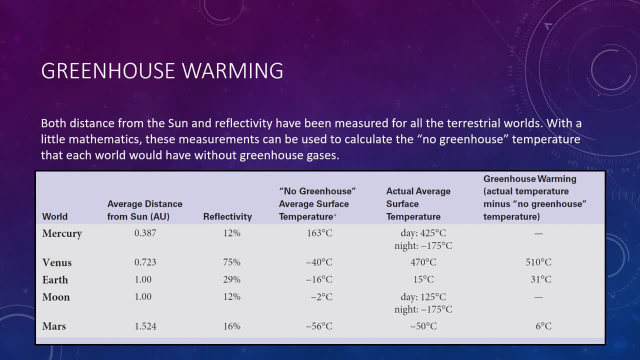 first, what we're going to take a look at is the structure of Earth's atmosphere and the Earth's magnetic field, And then we will go into the atmospheres of the other terrestrial worlds, So that being the moon and the other terrestrial planets, And then we'll come back and discuss. 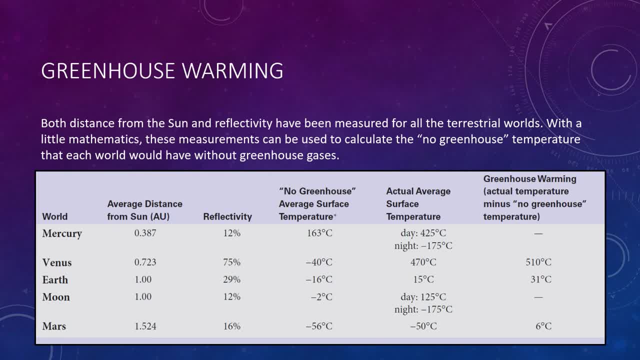 the general idea behind Earth's atmospheric history, how we came to our atmosphere today and then what we might be doing to it. So I look forward to talking to you guys. I look forward to talking to you in those videos, And we're getting close to concluding.